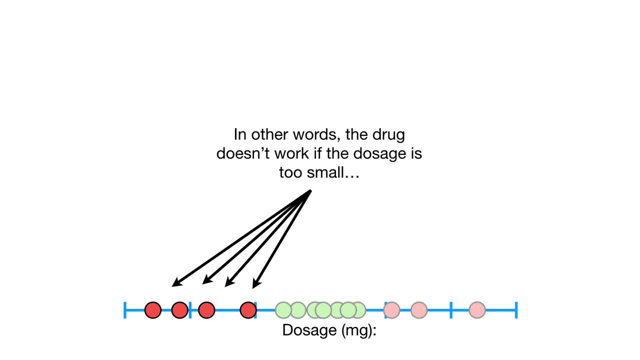 In other words, the drug doesn't work if the dosage is too small or too large. It only works when the dosage is too small or too large. It only works when the dosage is just right. Because this training dataset had so much overlap, we were unable to find a satisfying 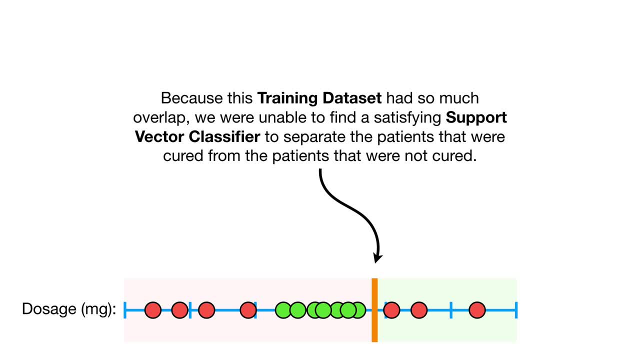 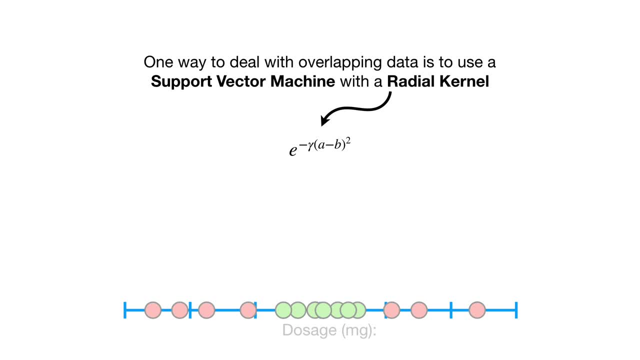 support vector classifier to separate the patients that were cured from the patients that were not cured. One way to deal with overlapping data is to use a support vector machine with a radial kernel, aka the radial basis function, RBF, Because the radial kernel finds support vector classifiers in infinite dimensions. it's not. 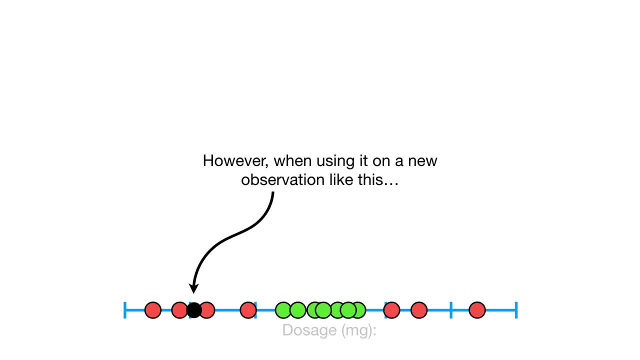 possible to visualize what it does. However, when using it on a new observation like this, the radial kernel behaves like a weighted nearest neighbor model. In other words, the closest observations, aka the nearest neighbors, have a lot of influence on how we classify the new observation. 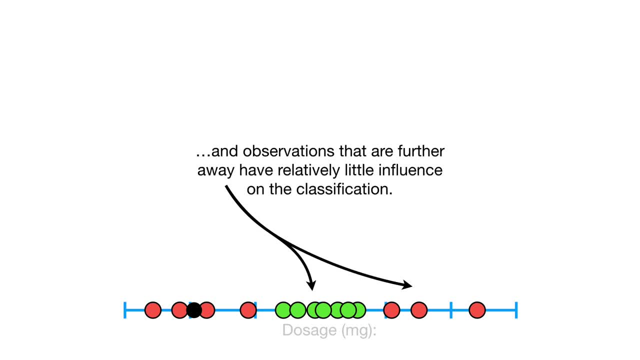 In other words, the closest observations, aka the nearest neighbors, have a lot of influence on how we classify the new observation, And the observations that are further away have relatively little influence on the classification. So since these observations are the closest to the new observation, the radial kernel- 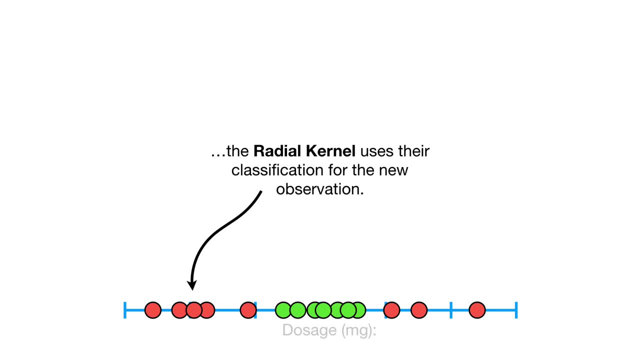 uses their classification for the new observation. Now let's talk about how the radial kernel determines how much influence each observation in the training dataset has on classifying new observations, Just like with the polynomial kernel. A and B refer to two different dosage measurements. 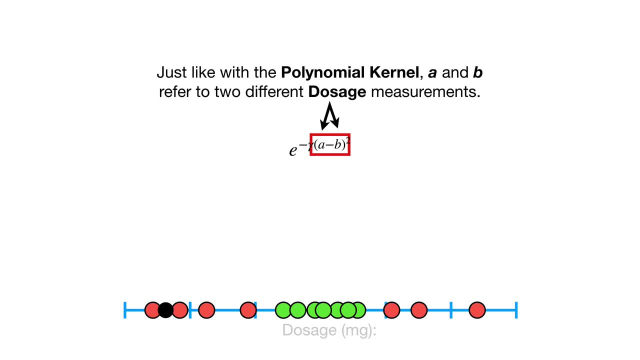 A and B refer to two different dosage measurements. The difference between the measurements is then squared, giving us the squared distance between the two observations. Thus, the amount of influence one observation has on another is a function of the squared distance Gamma, which is determined by cross-validation scales. the squared distance between the two. 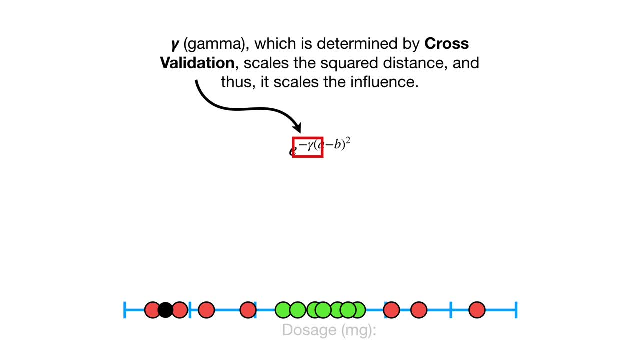 observations, and thus it scales the influence. For example, if we set Gamma equal to 1 and plug in the dosages from two observations that are relatively close to each other and do the math, we get 0.11 when Gamma equals 1.. 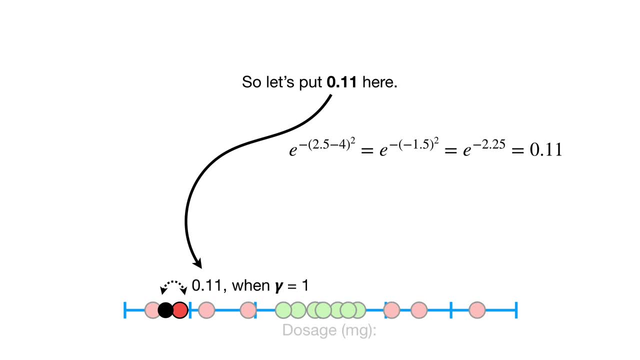 So let's put 0.11 here. Now let's set Gamma equal to 2 and plug in the same two dosages as before and do the math: When Gamma equals 2, we get 0.01,, which is less than when Gamma equals 1.. So we see that by scaling the distance, 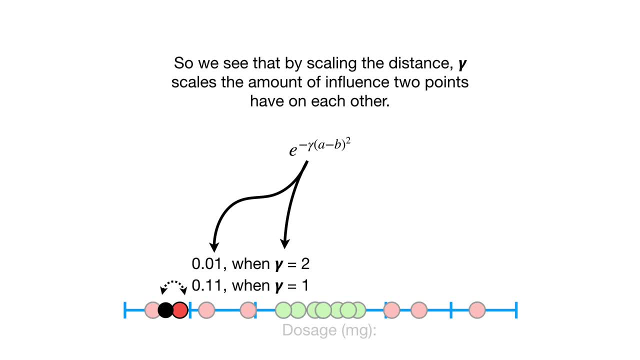 Gamma scales the amount of influence and Gamma scales the distance. So we see that by scaling the distance, Gamma scales the amount of influence two points have on each other. Small bam. Now let's set Gamma equal to 1 again and determine how much influence two observations have when they are. 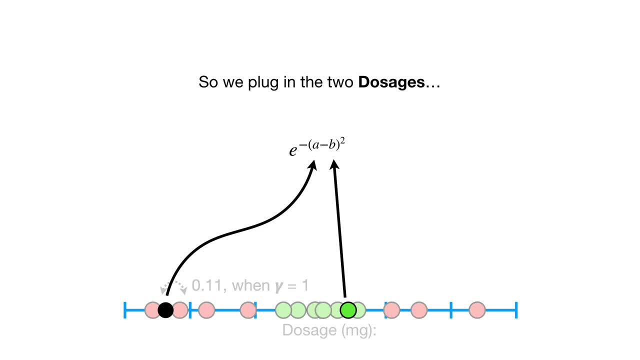 relatively far from each other. So we plug in the two dosages, do the math, and when the points are relatively far from each other, we get a number very close to 0. Thus the further two observations are from each other, the less influence they have on each other. 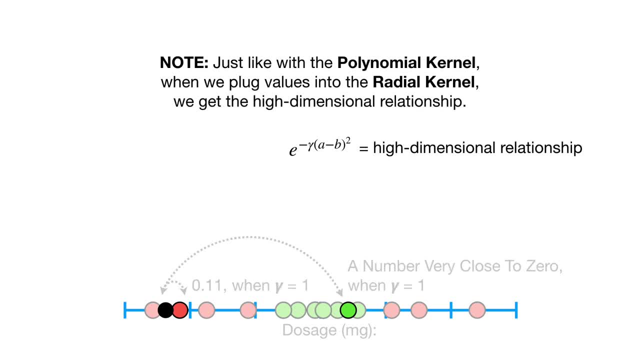 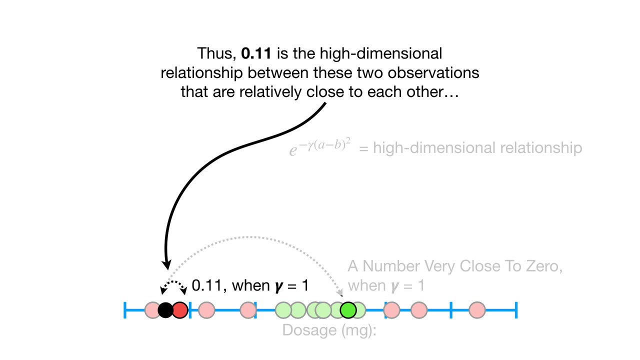 Note: just like with the polynomial kernel, when we plug values into the radial kernel we get the high-dimensional relationship. Thus, 0.11 is the high-dimensional relationship between these two observations that are relatively close to each other, and a number very close to 0 is the 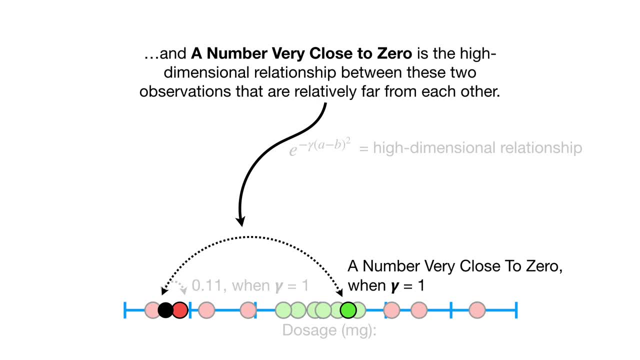 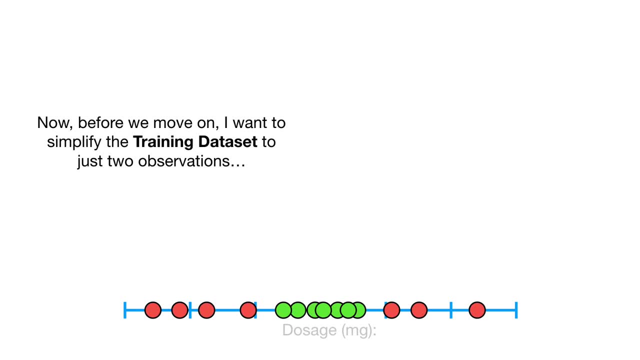 high-dimensional relationship between these two observations that are relatively far from each other: Medium bam. Now, before we move on, I want to simplify the training data set to just two observations and use the polynomial kernel to give us intuition into how the radial kernel works in infinite dimensions. When r equals 0, the polynomial kernel simplifies. 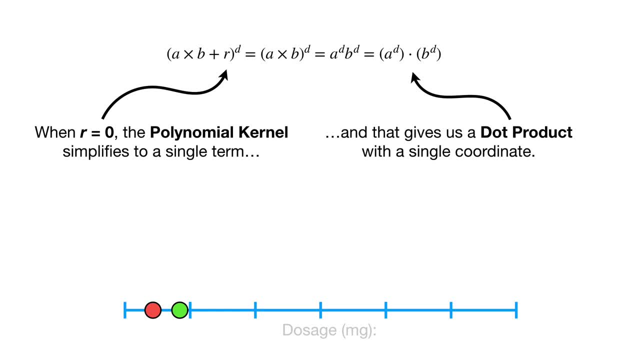 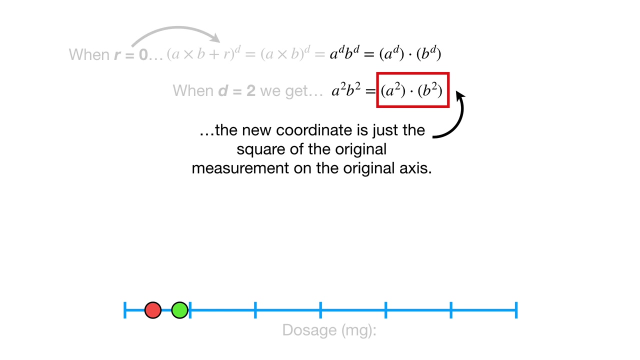 and that gives us a dot product with a single coordinate. When d equals 2, we get a squared times b squared, which is equal to the dot product of a squared and b squared. Since this dot product only has one coordinate, the new coordinate is just the square of the original measurement. 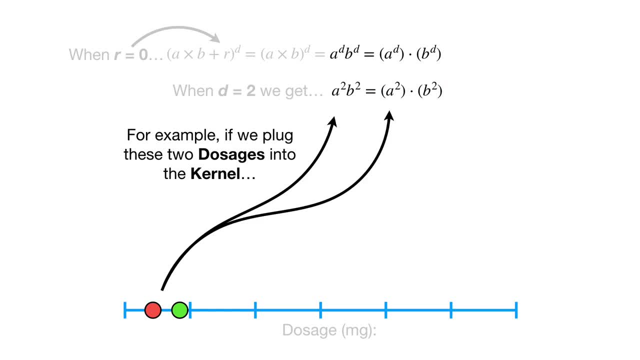 on the original axis. For example, if we take the original measurement of the original axis, if we plug these two dosages into the kernel, we get this dot product and that means the new axis coordinate for this point is 2.5 squared, which equals 6.25, and the new. 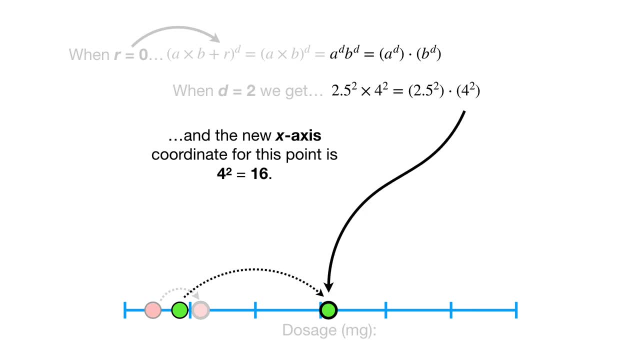 x axis. coordinate for this point is 4 squared, which equals 16.. In other words, when r equals zero and d equals 2, all the polynomial kernel does is shift the data to another field. After this analysis becomes complete, we can compute 真的温度 shipping officials to calculate the new Manhattan gradient. 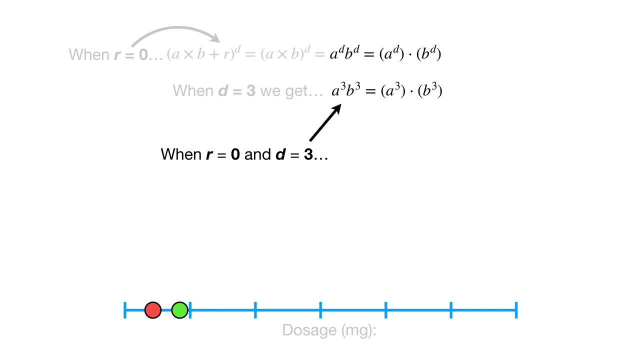 down the original axis. When r equals 0 and d equals 3,, we still only have one coordinate in the dot product and we shift the data down the x-axis further, because now we are cubing each value. Lastly, when r equals 0 and d equals 1,, 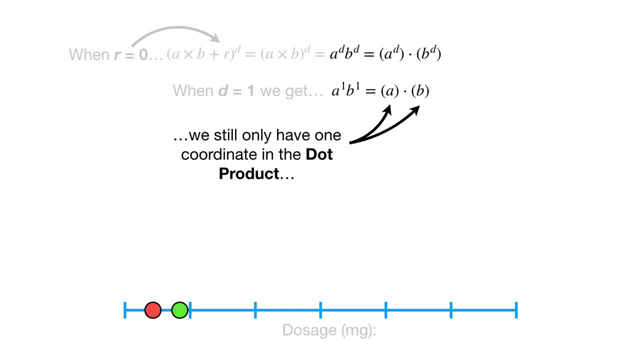 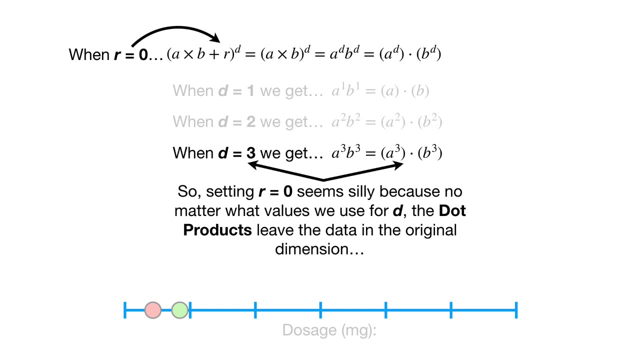 we still only have one coordinate in the dot product, but now the data just stays in its original location. So setting r equals 0 seems silly, because no matter what values we use for d, the dot products leave the data in the original dimension. 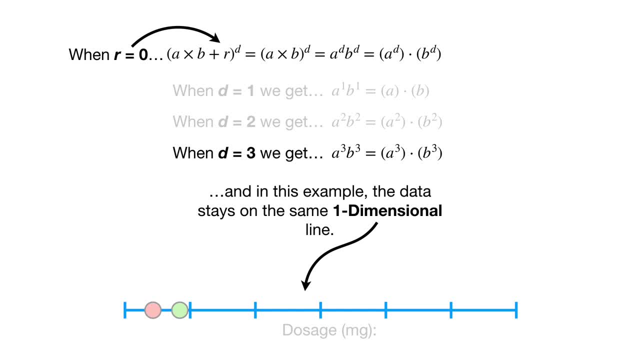 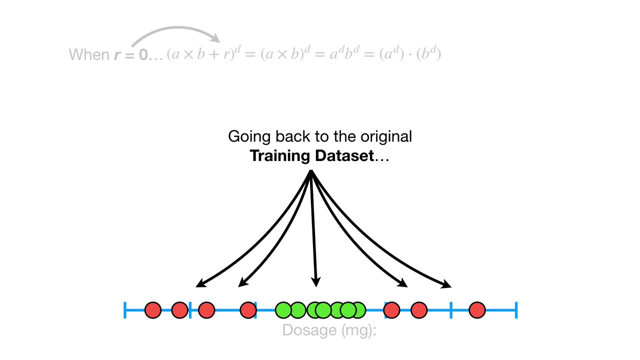 And in this example the data stays on the same one-dimensional line. However, it turns out that setting r equals 0 can result in some pretty awesome stuff. Going back to the original training data set, let's talk about what happens if we take a polynomial kernel. 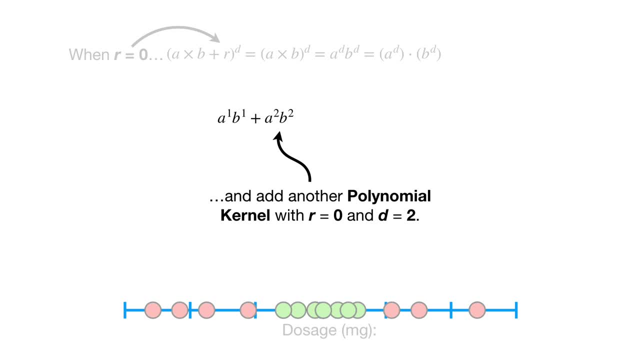 with r equals 0 and d equals 1, and add another polynomial kernel with r equals 0 and d equals 2. This gives us a dot product with coordinates for two dimensions. The first coordinate is the original dosage and the second coordinate is dosage squared. 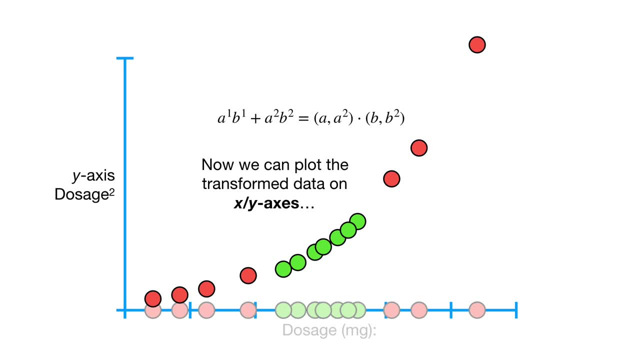 Now we can plot the transformed data on x-y axes and find a support vector classifier to separate the data. And by now you know that we don't actually do the transformation. We just solve for the dot product to get the high-dimensional relationships. 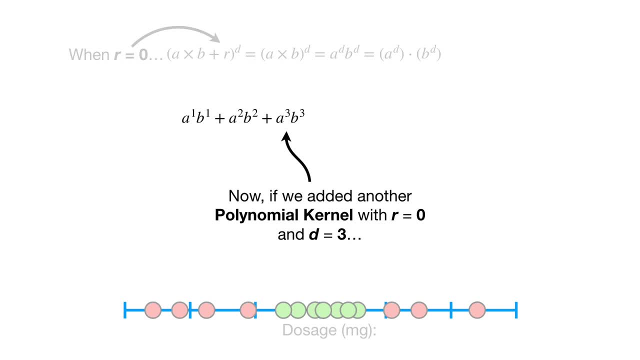 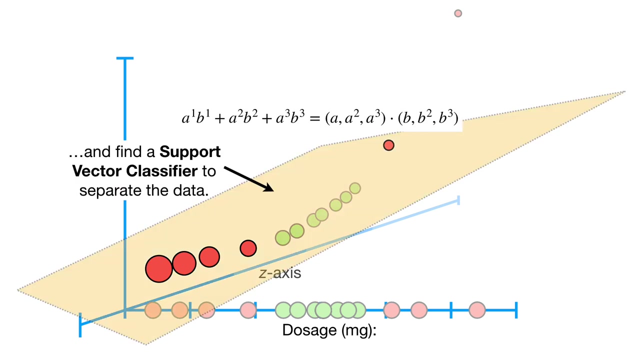 Now if we added another polynomial kernel with r equals 0 and d equals 3, then the dot product will be the same. The dot product has coordinates for three dimensions and we can plot the transformed data on x-y-z axes and find a support vector classifier to separate the data. 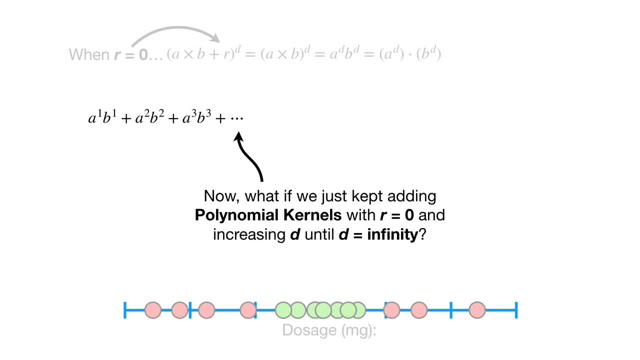 Now what if we just kept adding polynomial kernels, with r equals 0 and increasing d until d equals infinity? That would give us a dot product with coordinates for an infinite number of dimensions. That would be awesome, right? Well, that's exactly what the radial kernel does, so let's talk about it. 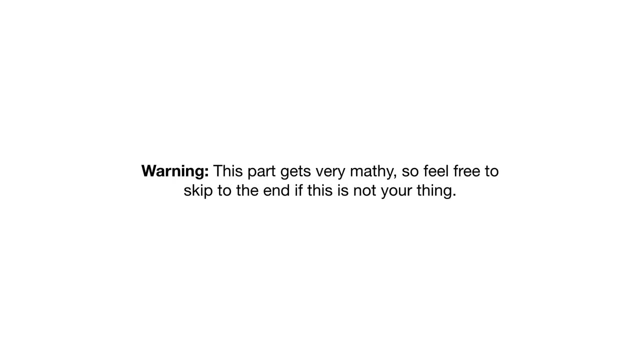 Warning: this part gets very mathy, so feel free to skip to the end. if this is not your thing, Let's start with the radial kernel and multiply out the square: Beep boop, boop, beep boop. 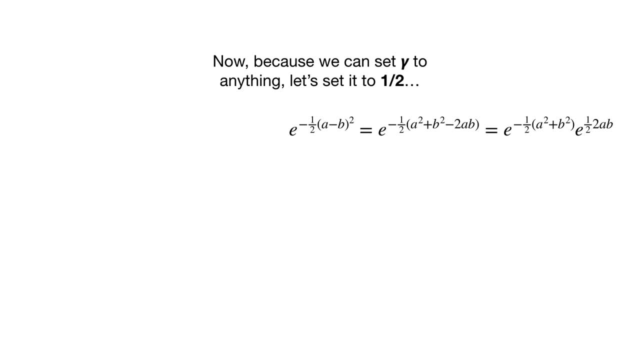 Now, because we can set gamma equal to anything. let's set it to 1: half, So that this 2 goes away. Now let's create the Taylor series expansion of this last term. Wait a minute. what's a Taylor series expansion? 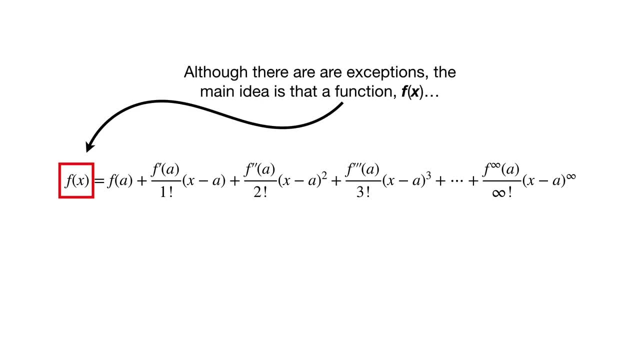 This big thing is a Taylor series. Although there are exceptions, the main idea is that a function f of x can be split into an infinite sum. Since this is very abstract, I'm going to give it a name: Very abstract. let's walk through how to convert e to the x into an infinite sum. 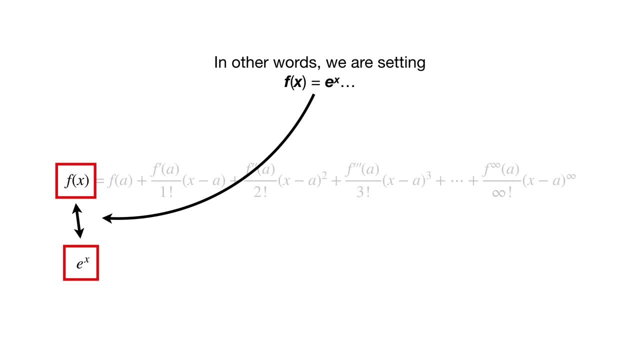 In other words, we are setting f of x equal to e to the x, And that means f of a equals e to the a. Now we plug in the derivative of e to the x, evaluated at a divide by 1 factorial and multiply by x minus a. 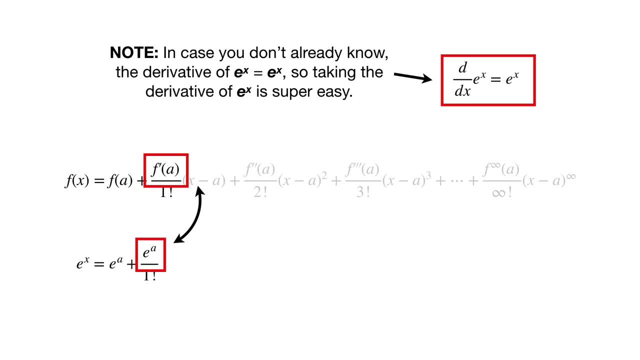 Note: In case you don't already know, the derivative of e to the x equals e to the x, So taking the derivative of e to the x is super easy. Now we plug in the second derivative of e to the x, evaluated at a divide by 2 factorial. 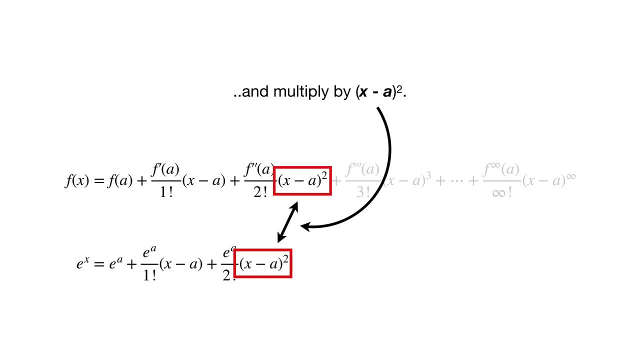 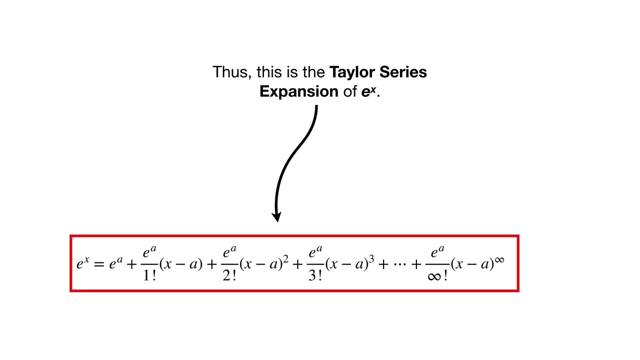 and multiply by x minus a squared, Then we keep adding terms based on higher derivatives until we get to infinity. Thus this is the Taylor series expansion of e to the x. Now he question is: what is a? The Taylor series says that a can be any value as long as f of a exists. 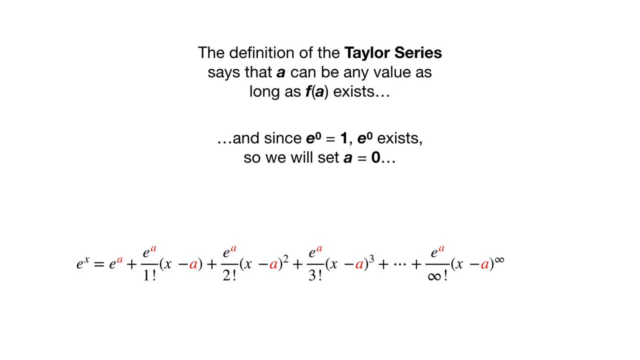 Since we justify a, we use f of a on both sides and give a %a. Since e to the zero equals 1, it will be a нее that exists. E to the zero exists, We will set a equal to zero. Now, f of a means f of a to be million, and since f of a is 0. It is such that if f of a is 1, then it's a million, and since f of a means 0, then x equals 0.. 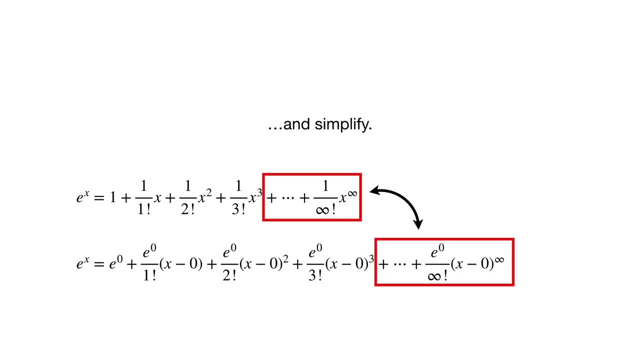 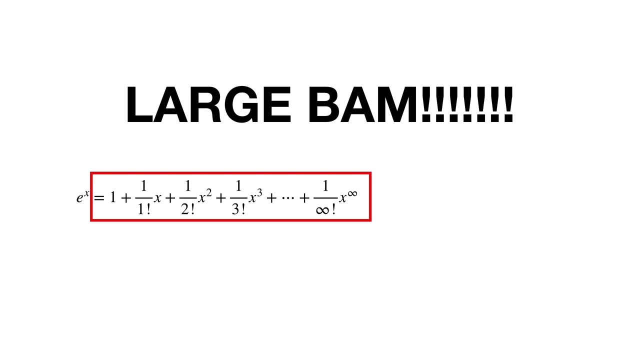 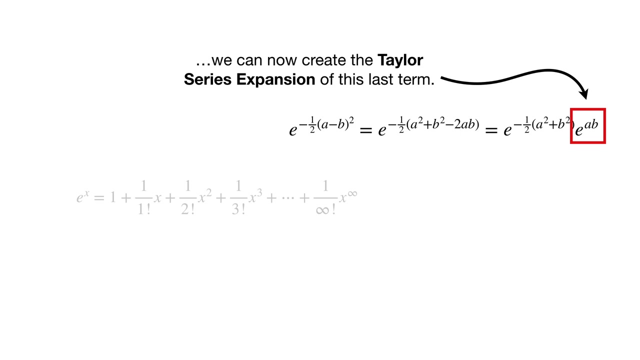 simplify. Thus, if we can accept that the Taylor series expansion does what it says it does- e to the x is equal to this infinite sum, Large BAM Going back to the radial kernel- we can now create the Taylor series expansion of this last term. 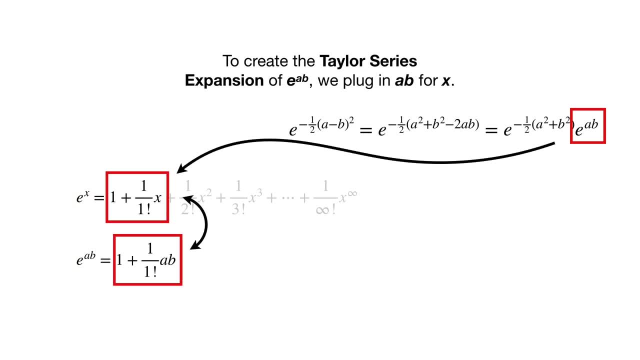 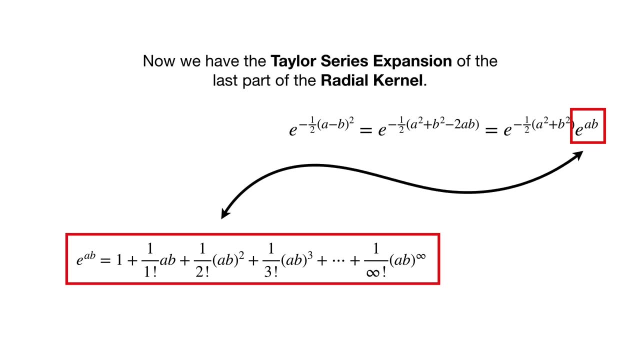 To create the Taylor series expansion of e to the ab. we plug in ab for x. Now we have the Taylor series expansion of the last part of the radial kernel. Okay, time to take a deep breath. We've done a lot, but we still have a few more steps before. 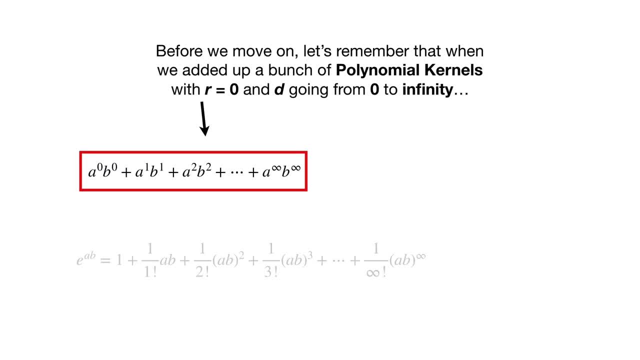 we are done and get to eat snacks. Before we move on, let's remember that when we added up a bunch of steps, we still have a few more steps to do, So let's take a deep breath. and a bunch of polynomial kernels: with r equals 0 and d going from 0 to infinity, We got a dot product. 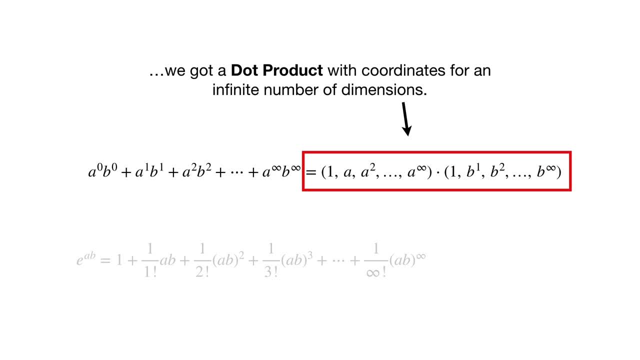 with coordinates for an infinite number of dimensions. Now observe that a polynomial kernel with r equals 0 and d equals 0 is equal to 1.. And a polynomial kernel with r equals 0 and d equals 1 is equal to a times b. And a polynomial kernel with r equals 0 and d equals 1 is equal to. 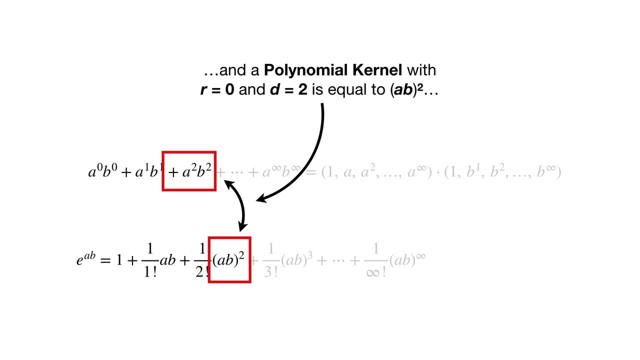 a times b, squared, Etc, etc. etc. Thus, each term in this Taylor series expansion contains a polynomial kernel, with r equals 0 and d going from 0 to infinity. Now, just to remind you, converting this sum to a dot product was easy. 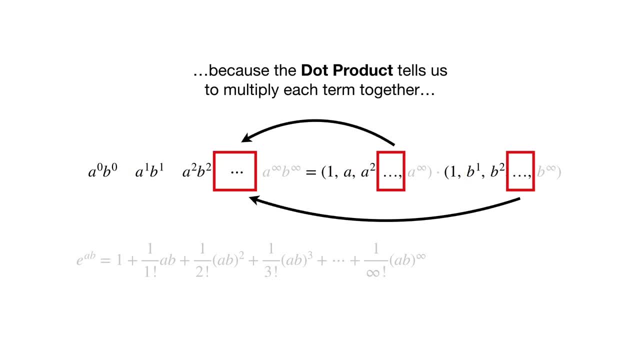 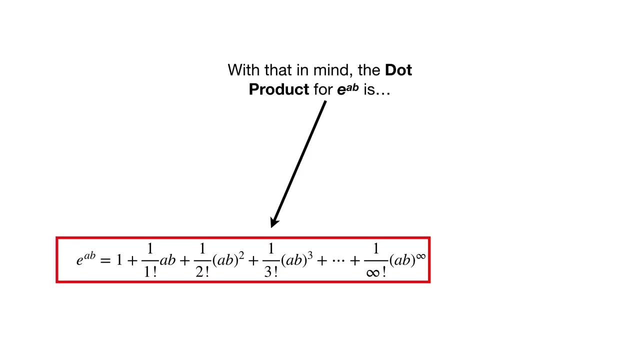 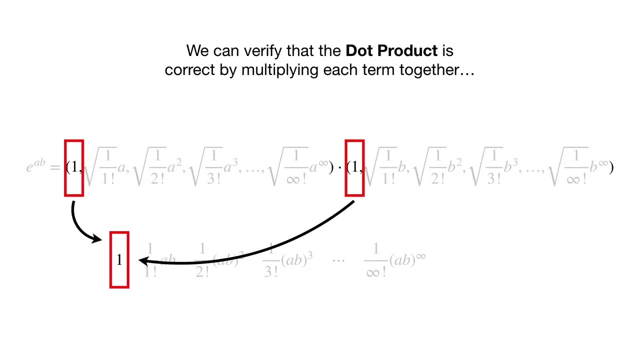 Because the dot product tells us to multiply each term together and then add up all the terms With that in mind. the dot product for e to the ab is this: We can verify that the dot product is correct by multiplying each term together and add up the new terms to get the Taylor series. expansion of e to the. 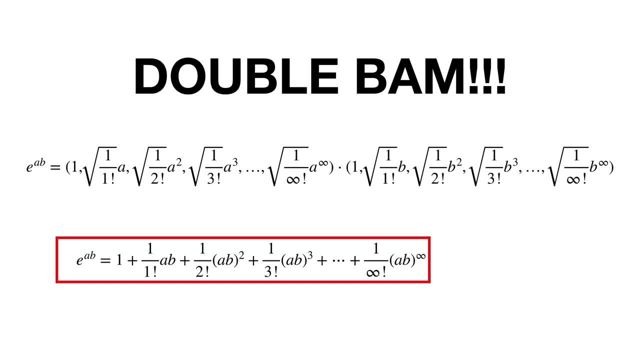 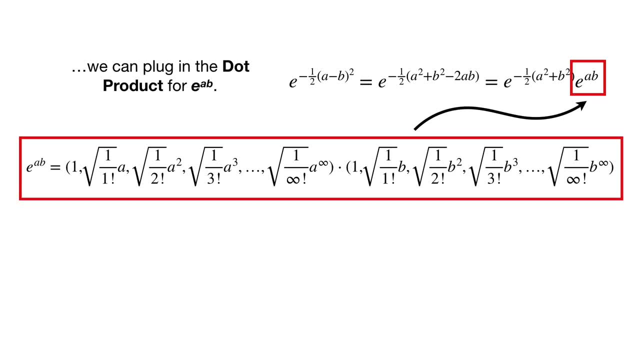 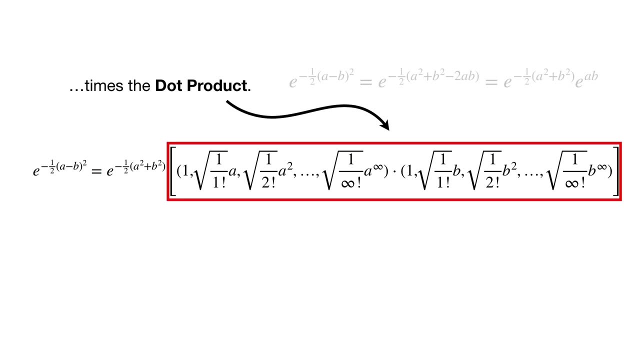 ab, Double bam. Going back to the original radial kernel, we can plug in the dot product for e to the ab. Now the radial kernel is equal to this term times the dot product. To make the radial kernel all one dot product instead of something times a dot product. 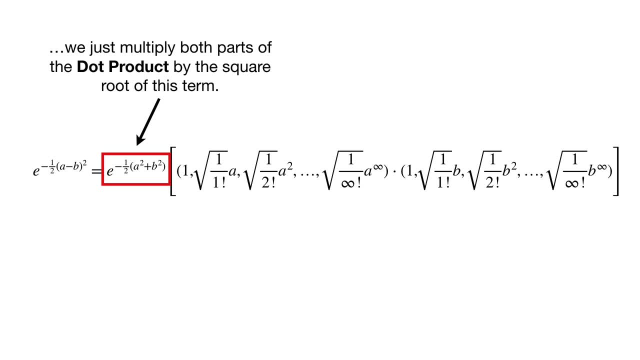 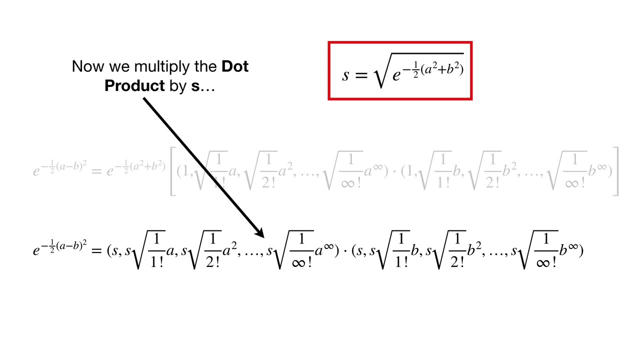 we just multiply both parts of the dot product by the square root of this term, So we can fit everything onto the screen. let's, let s equal the square root of the first term. Now we multiply the dot product by s And at long last we see that the radial kernel is equal to a dot. 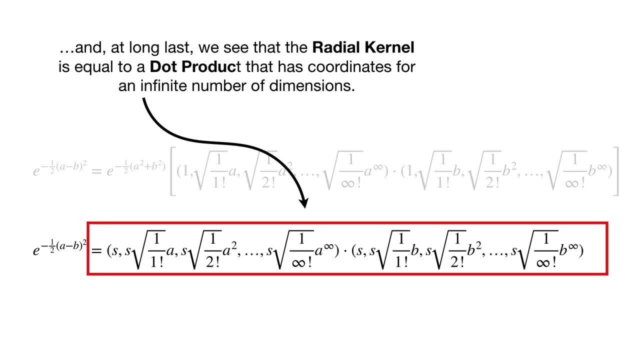 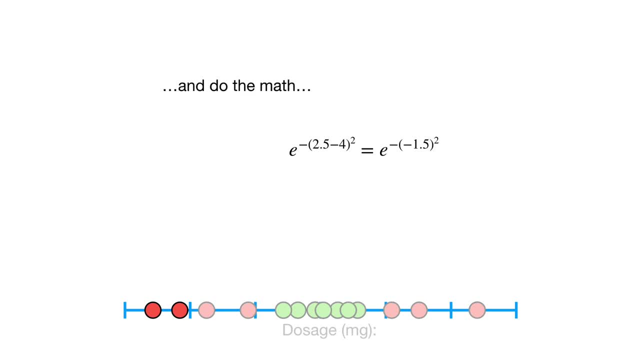 product that has coordinates for an infinite number of dimensions. That means when we plug numbers into the radial kernel and do the math, the value we get at the end is the relationship between the two points in infinite dimensions. Triple bam, Now we can go eat snacks. Hooray, We've made it. 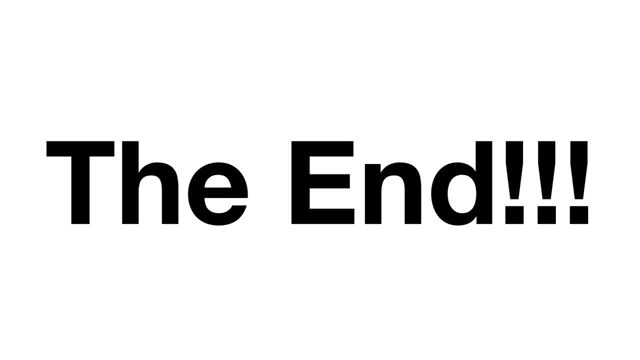 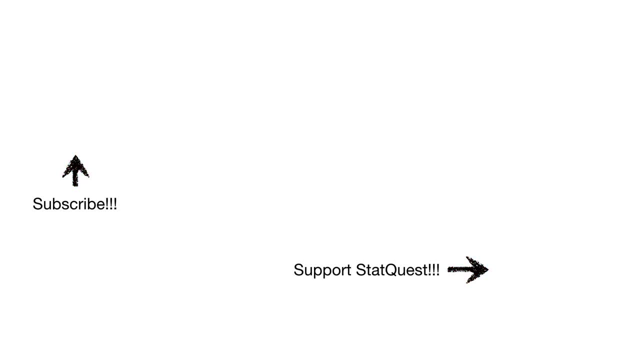 to the end of a simple math lesson, Here's another exciting StatQuest. If you like this StatQuest and want to see more, please subscribe. And if you want to support StatQuest, consider contributing to my Patreon campaign, becoming a channel member, buying one or two of my